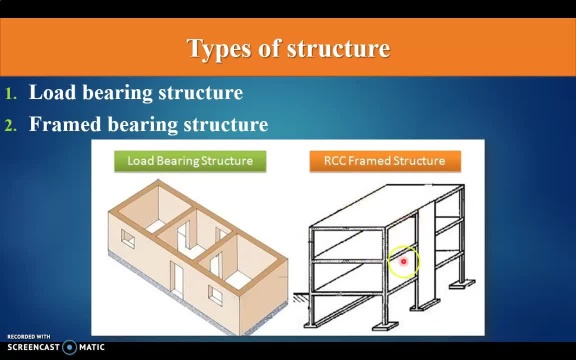 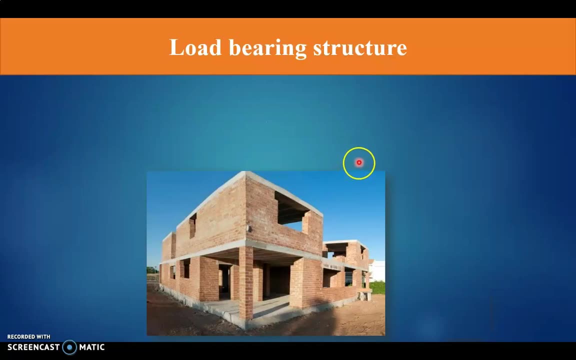 Second is a rcc frame structure. In rcc frame structure all the structure members are involved, like beam, column, slabs and footing. So these all types of structure member are involved in the building a frame type of structure. okay, So let's move about. first of all, understand about 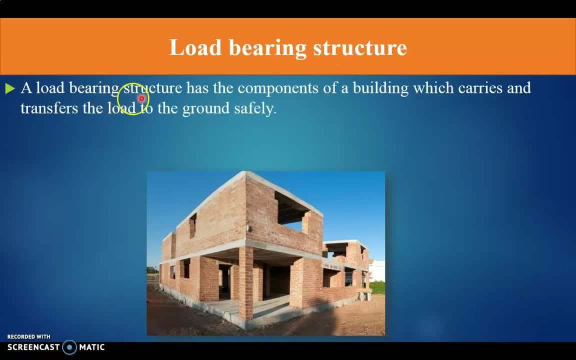 load bearing structure. The load bearing structure. Load bearing structure has the components of a building. Load bearing structure has the components of a building. Load bearing structure, which is the standard part of a building, and the components of the structure building which carries and transfer the load to the ground safely. and this structure guarantee. 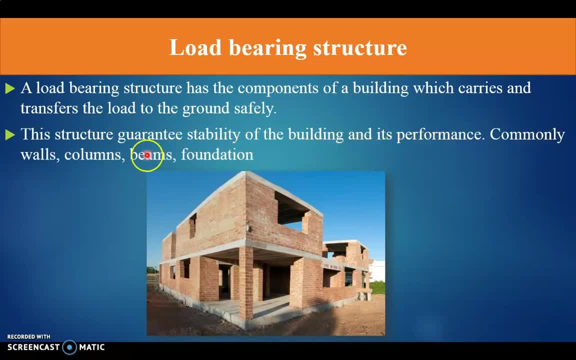 stability of the building and its performance. commonly, walls, column beam and foundations are to be carry all the loads. so in this picture you can see in the column here the walls to be constructed as a column, okay, and all the types you can see in this, all the sides of all the. 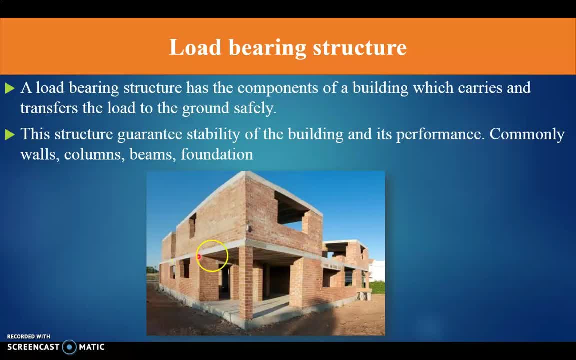 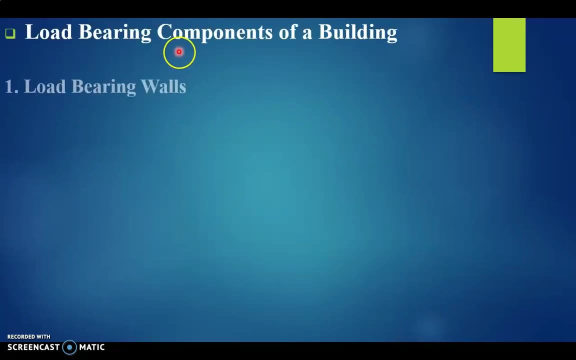 walls to be construction and, in the upper level, total slab to be provided. this type of structure is called the load bearing structure and its limitation to construct is maximum two store building to be construct in this type of structure. then, after load bearing components of a building, load bearing walls transfer the loads from slabs above it to the foundation and these walls can be. 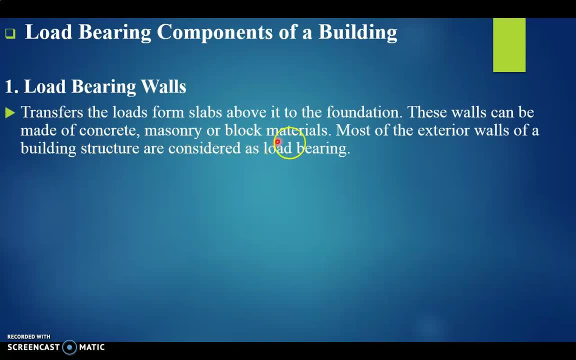 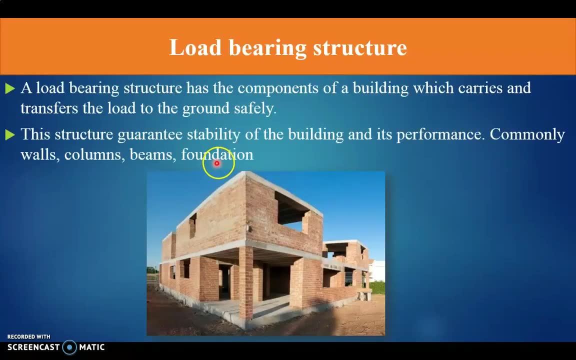 made of concrete, masonry or block materials. most of the exterior walls of a building structure are considered as a load bearing, so in this picture you can also see how the walls to be as a play role in the load bearing structure and carry all the slabs load to the foundations. then, after any load bearing wall should have minimum thickness. 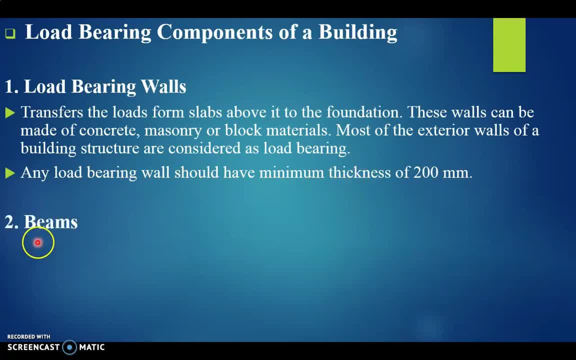 of 200 mm. next is a beam, primary load bearing components of a structure which can be made from wood, concrete or metal. the capacity of load bearing depends on the depth and width of the beam, so the how the total stores to be construction in the load bearing structure, it depends on the 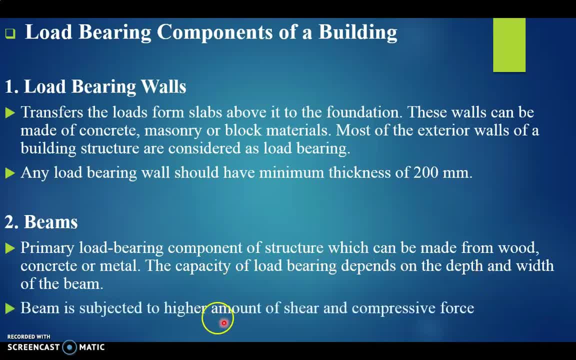 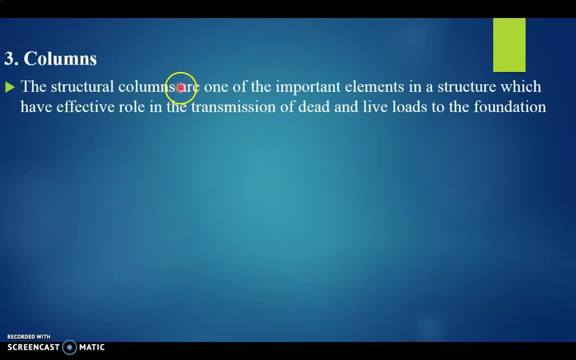 depth and width of the beam and beam is subjected to higher amount of shear and the compressive force. then after understand about column using in the load bearing structure. so the structural column are one of the important element in structure which have effective role in the transmission of the load bearing structure. so the structural column are one of the important. 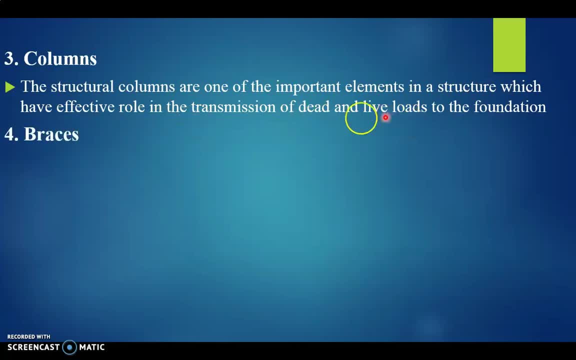 elements in structure which have effective role in the transmission of dead load and live load to the foundation. but in load bearing structure mainly columns are built up as a normally in the wall construction. okay, second is a braces. braces are structural element used in the framework structural system. this load bearing elements helps in stiffening the framework effectively. 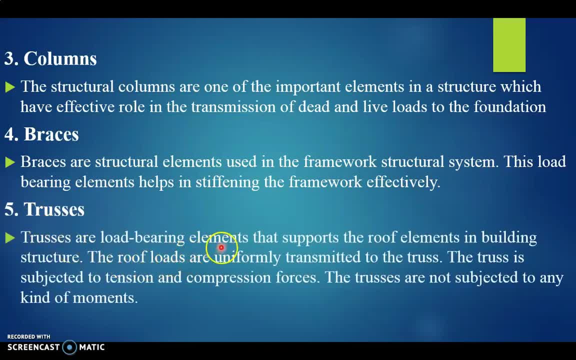 thereafter understand about truss. truss are load bearing element that support the roof elements in the building structure. the roof loads are uniformly transmitted to the truss and the truss is subjected to tension and compression forces. the trusses are not subjected to any kind of moment. these type of trusses are. 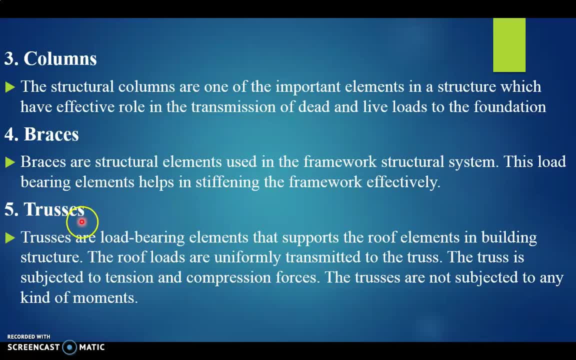 mainly using in the roof area, okay, so when the walls to be constructed in the slabs, in the slab portion, trusses are to be provided, okay, and the root load are uniformly transmitted to the truss and the truss is subjected to tension and compression forces to be carried. 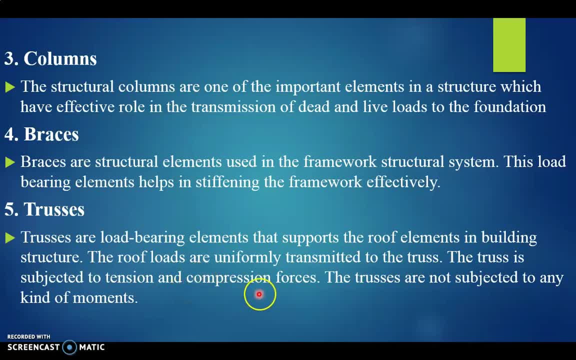 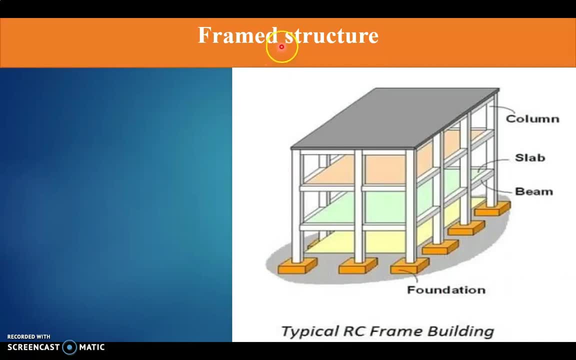 and they carry only loads, not carry any type of moment let's understand about. second type of structure is a frame structure in the frame structure. in this picture you can see the foundations, the beam and slab and the column and the upper layered slab. okay, this all the structural. 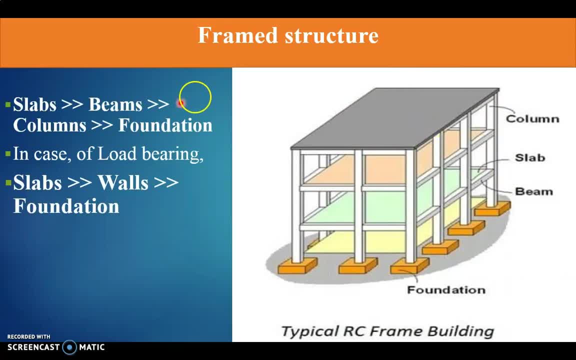 members are involved in the frame bearing structure. so here, slabs transfer all the loads to the beam beam transfer, wall loads to the column beam transfer all beautiful load, so later theirs. so in this particular case, i am drawing the diagram of the frame structure and this will be transparent. and basically, it is very easy to understand that this structure is not designed with industrially careful, like the idea of structure which is not referring only to construction andальный, as it is not, its own painting would be completely impaired. so as we consider this first, I would 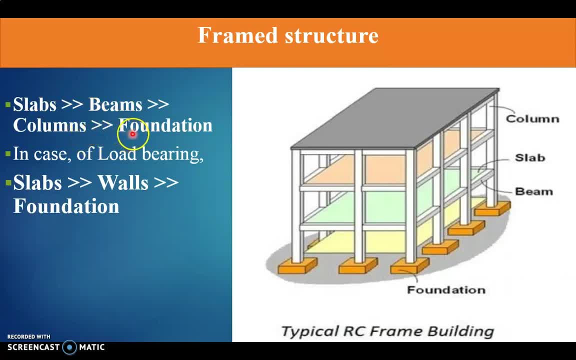 column and column transfer all the loads to the foundation. in the case of load bearing, slab transfer the load to the wall and wall transfer all the load to the foundation. so mainly difference. you can see that how the frame bearing structure involved in the four components and the load. 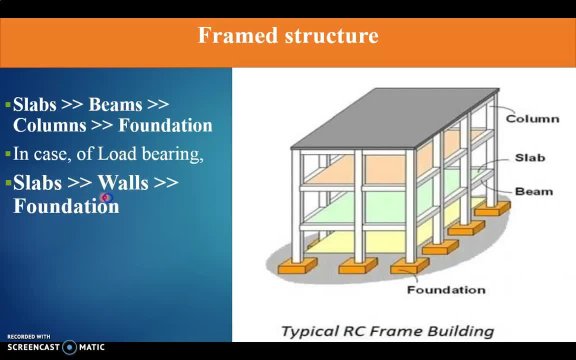 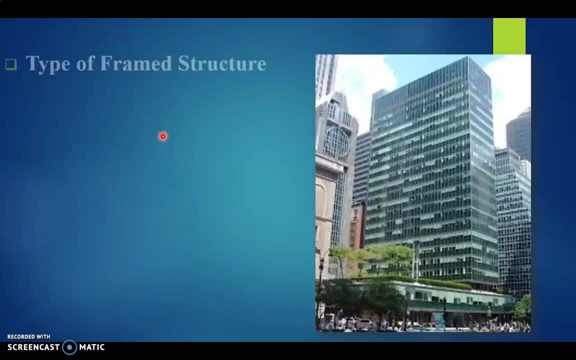 bearing structure involving only three components. that mean is a walls, okay, and in the frame structure, main component is a slab, beam, column and also foundation. let's understand about type of frame structure. first of all, digit frame structure. so in the digit frame structure these are built at the side and they provide more stability and resist rotations effectively. so in